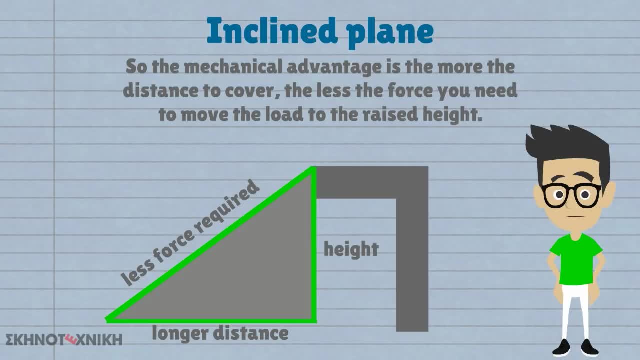 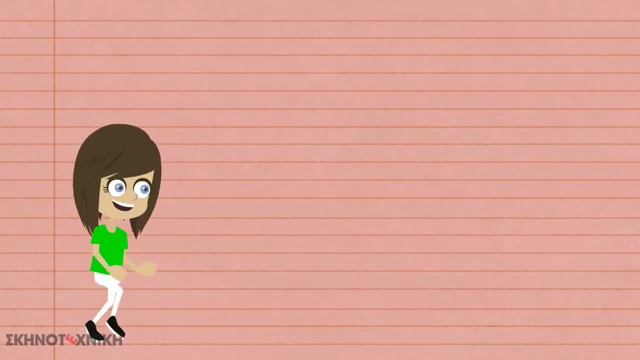 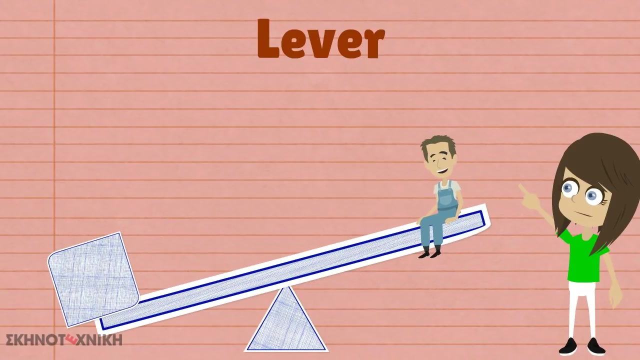 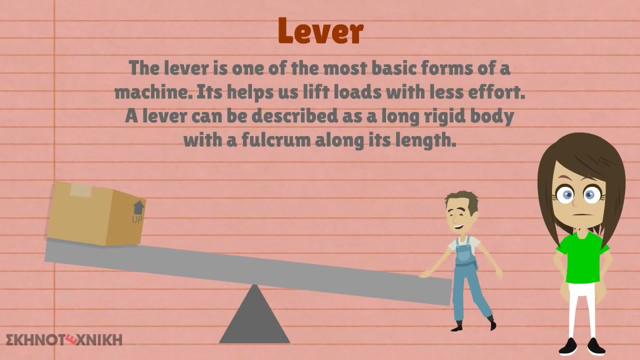 need to move the load. The lever is one of the most basic forms of a machine. It helps us lift loads with less effort. A lever can be described as a long, rigid body with a fulcrum along its length. A lever can be described as a long, rigid body with a fulcrum along its length. 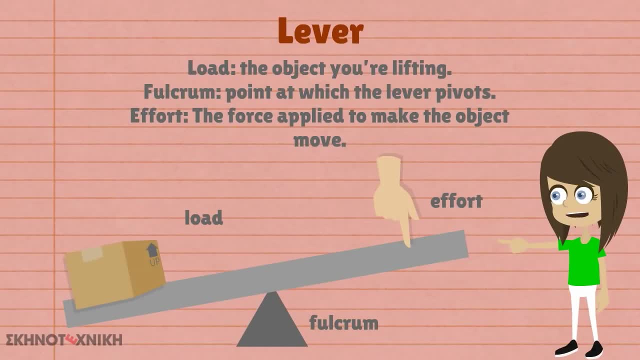 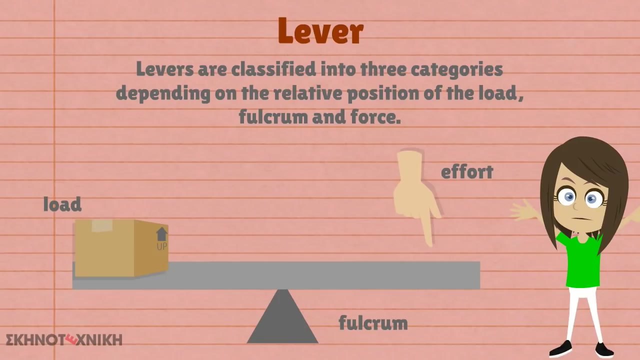 Common Park FOR현. Load the object you are lifting. Fulcrum point at which the lever pivots: Effort the force applied to make the object move. Top of the Class. Lovers are classified into 3 categories depending on the relative position of the load: the. 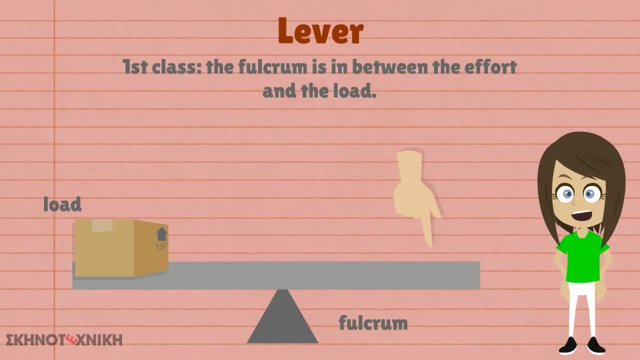 fulcrum and the force. In the first class, the fulcrum is in between the Effort and the Load. In the second class, the load is between the fulcrum and the Effort. In the second class, the load is between the fulcrum and the Effort. 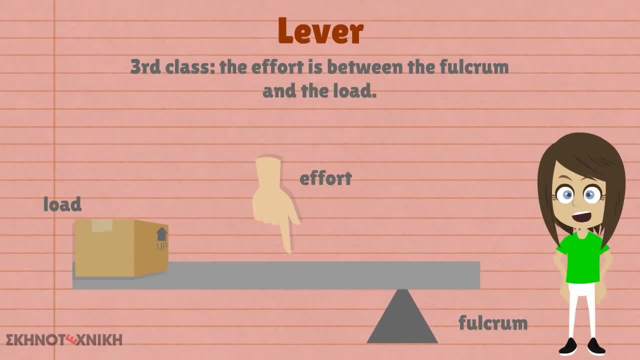 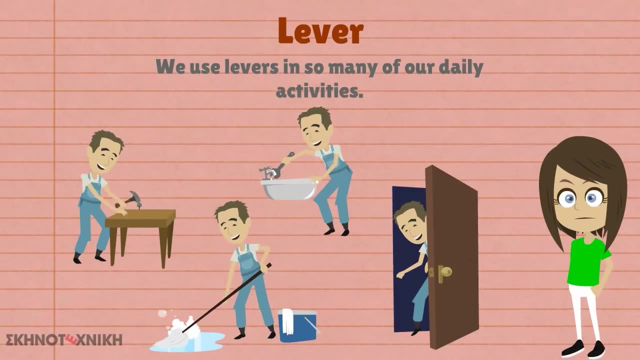 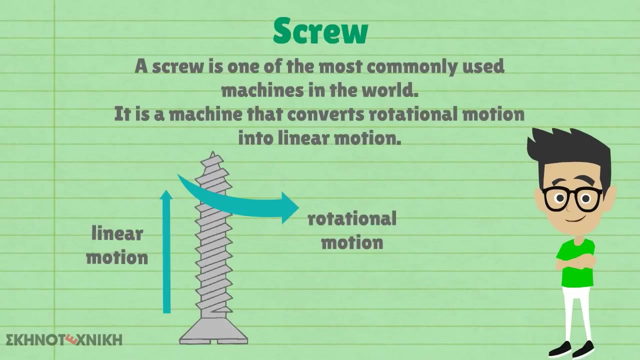 In the third class, the load is in between the fulcrum and the Effort, And in the third class, the effort is between the fulcrum and the load. We use levers in so many of our daily activities: Screw. A screw is one of the most commonly used machines. 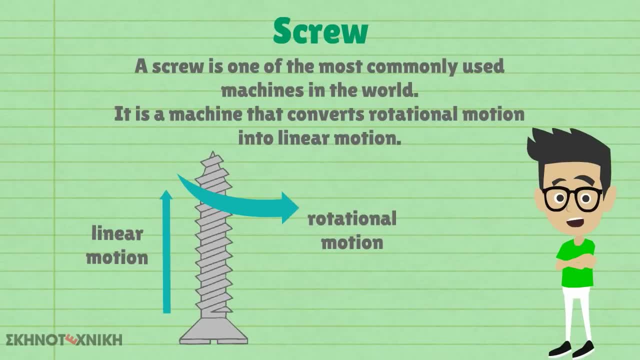 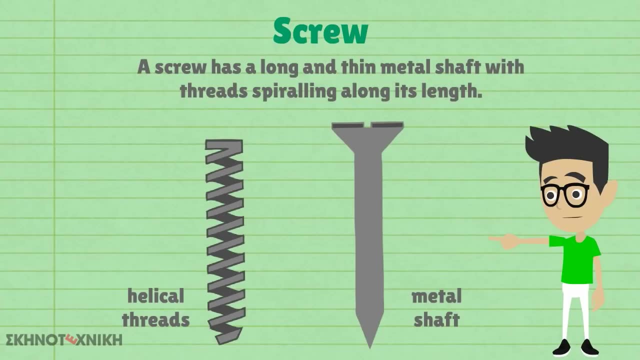 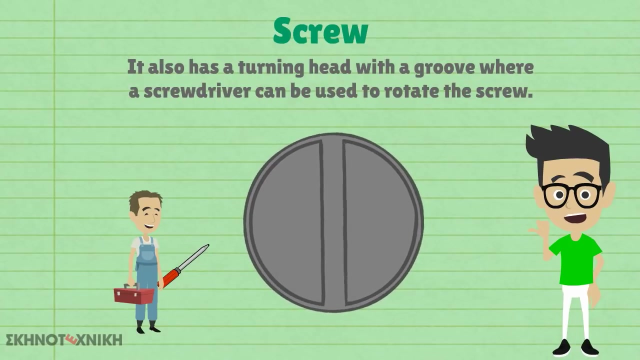 in the world. It is a machine that converts rotational motion into linear motion. A screw has a long and thin metal shaft with threads spiraling along its length. It also has a turning head with a groove where a screwdriver can be used to rotate the screw. 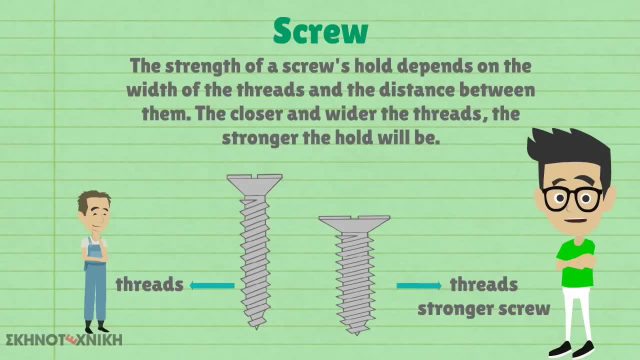 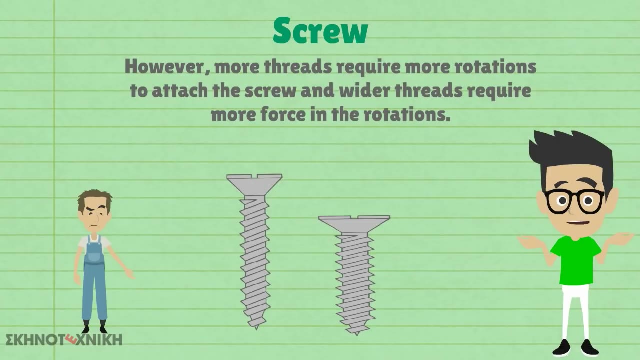 The strength of a screw's hold depends on the width of the threads and the distance between them. The closer and wider the threads, the stronger the hold will be. However, more threads require more strength, More rotations to attach the screw, and wider threads require more force in the rotations. 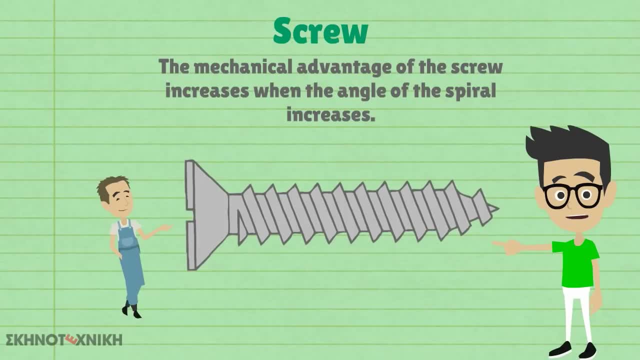 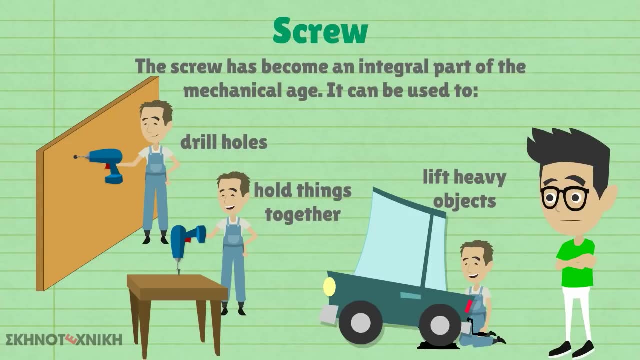 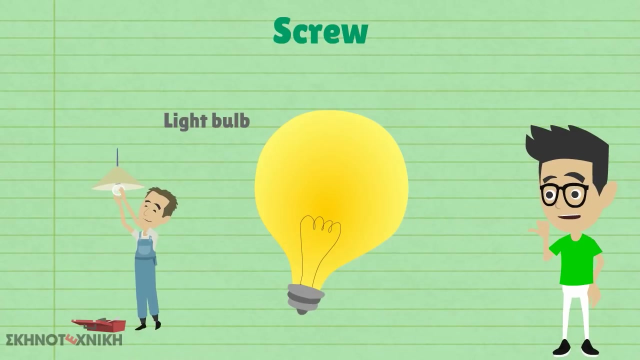 The mechanical advantage of the screw increases when the angle of the spiral increases. The screw has become an integral part of the mechanical age. It can be used to drill holes, hold things together and lift heavy objects. Did you know that a light bulb is an example of a screw? 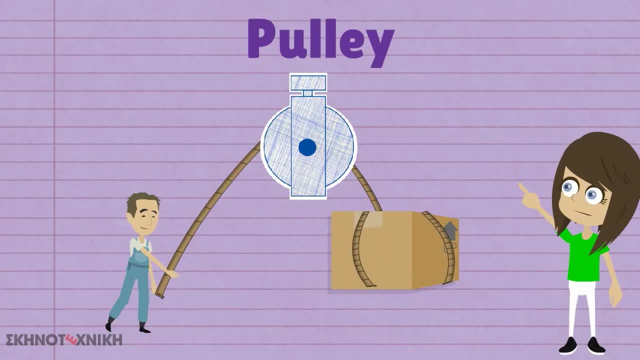 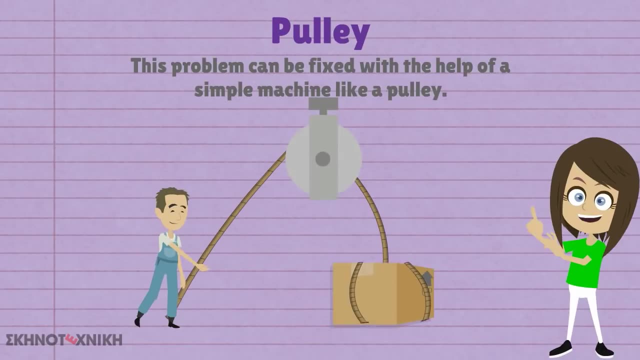 Finally, let's look at a simple machine that can hold heavy objects. A small machine can hold heavy objects with its long and thin threads, but not the small one. For example, a heavy object can hold heavy objects with only a single estimating force. 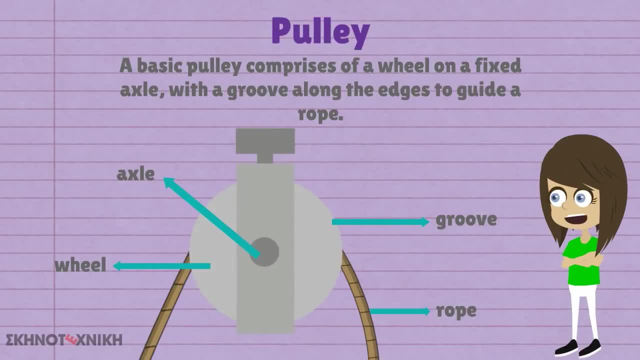 and it can hold only heavy objects with a single estimating force. This problem can be fixed with the help of a simple machine like a pulley. A basic pulley comprises of a wheel on a fixed axle with a groove along the edges to guide a rope. 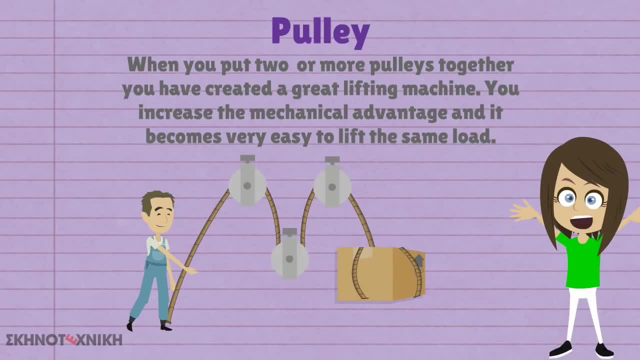 When you put two or more pulleys together, you have created a great lifting machine. Do you know what a lift machine looks like? Let us know in the comments. You increase the mechanical advantage and it becomes very easy to lift the same load. 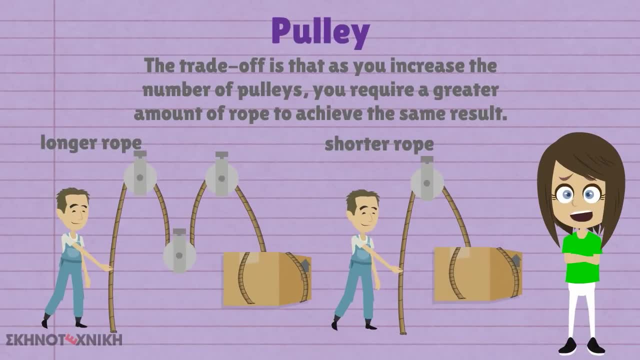 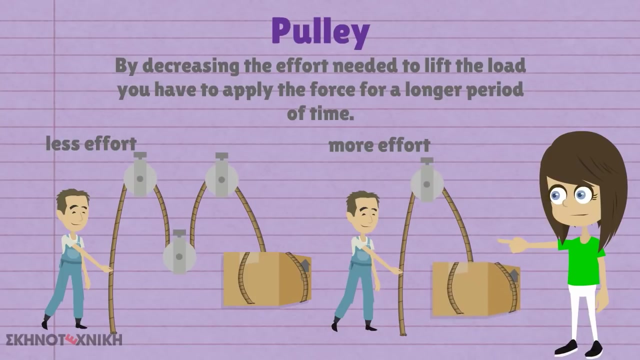 The trade-off is that as you increase the number of pulleys, you require a greater amount of rope. to achieve the same result By decreasing the effort needed to lift the load, you have to apply the force for a longer period of time. 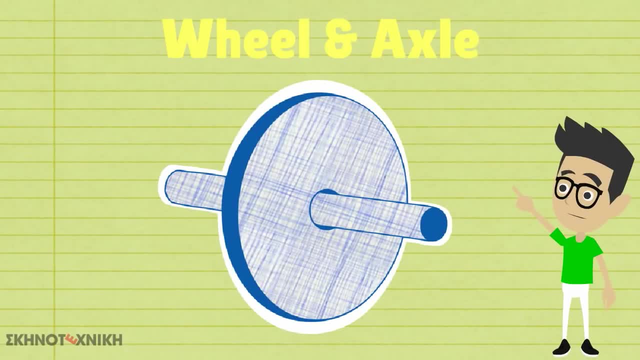 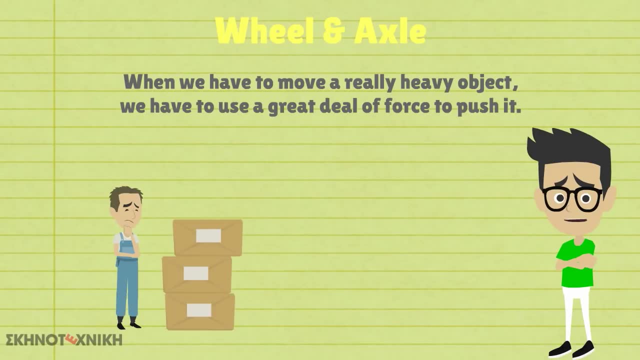 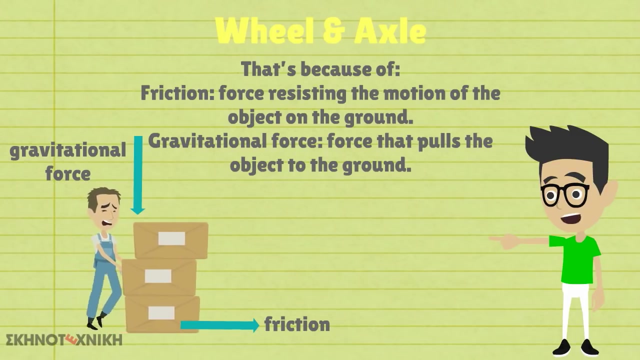 Wheel and axle. When we have to move a really heavy object, we have to use a great deal of force to push it. That's because of friction, the force that's resisting the motion of the object on the ground, And gravitational force, the force that pulls the object to the ground. 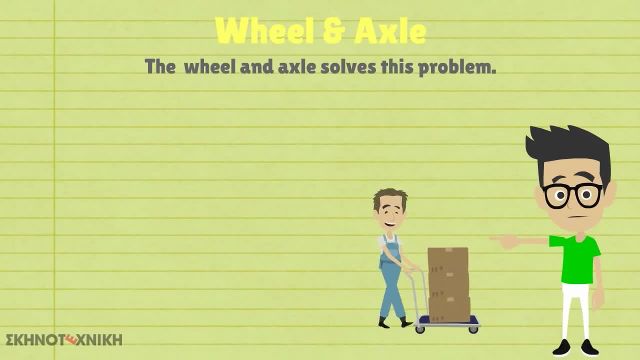 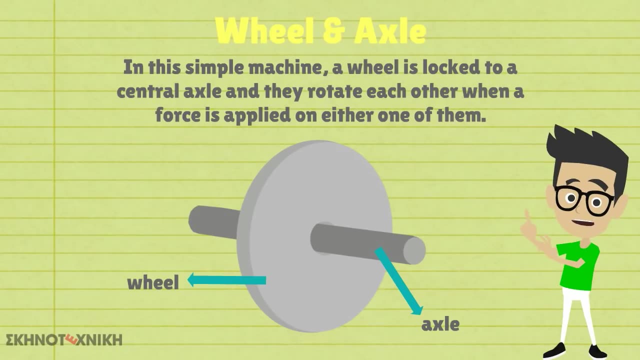 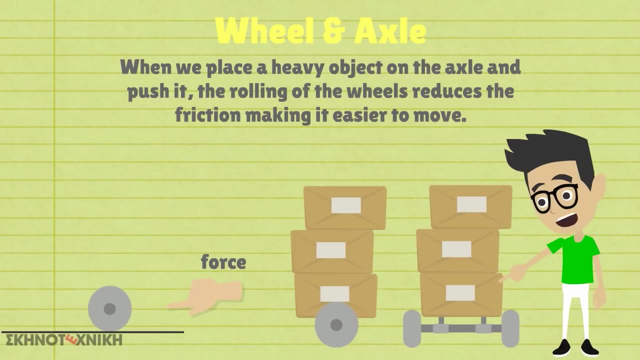 The wheel and axle solves this problem. Wheel and axle In this simple machine. a wheel is locked to a central axle and they rotate each other when a force is applied on either one of them. When we place a heavy object on the axle and push it, the rolling of the wheels reduces the friction, making it easier to move. 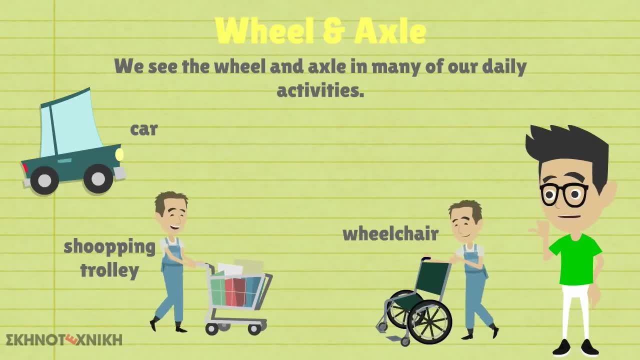 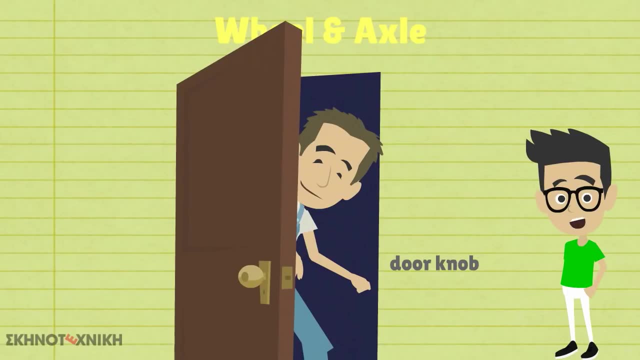 We see the wheel and axle in many of our daily activities, Such as when we use a car Wheel and axle, A shopping trolley or a wheelchair. Did you know that a door knob is an example of a wheel and axle? 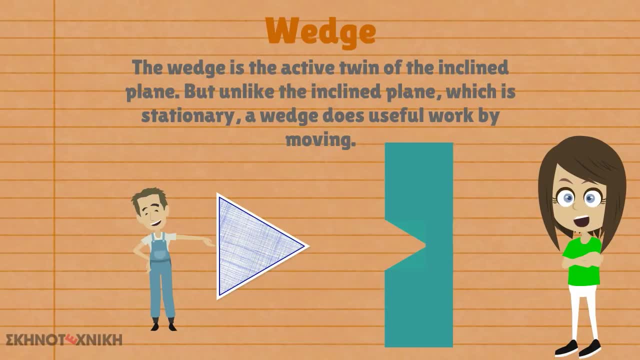 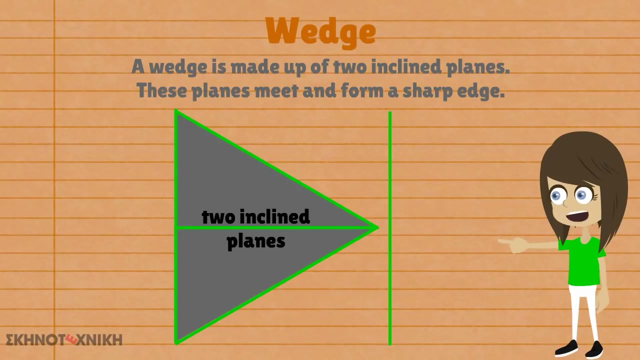 Wench. The wench is the active twin of the inclined plane. But unlike the inclined plane, which is stationary, a wench does useful work on moving. A wench is made up of two inclined planes. These planes meet and form a sharp edge.